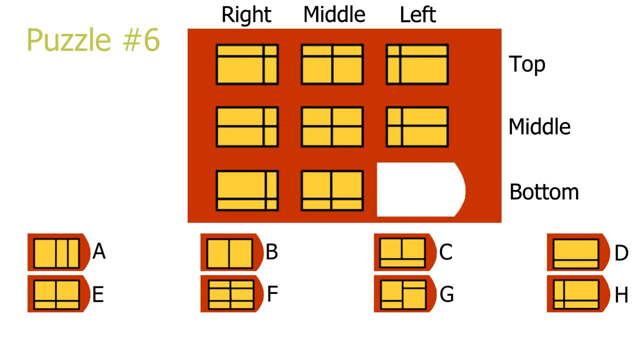 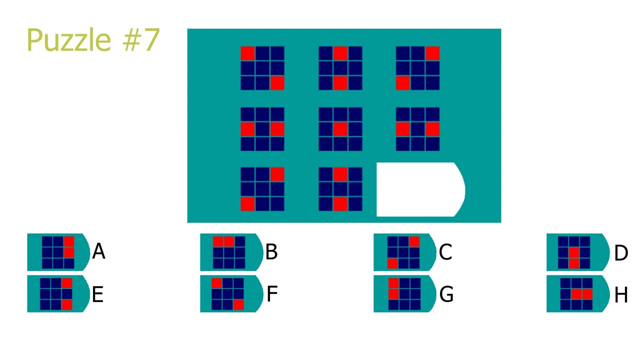 middle and left positions on the columns for the vertical line and top, middle and bottom positions on the rows for the horizontal line. This leads to a left vertical line, vertical line with a bottom horizontal line. H is correct. Puzzle 7.. Another row and column puzzle. This puzzle have two row and column elements, which 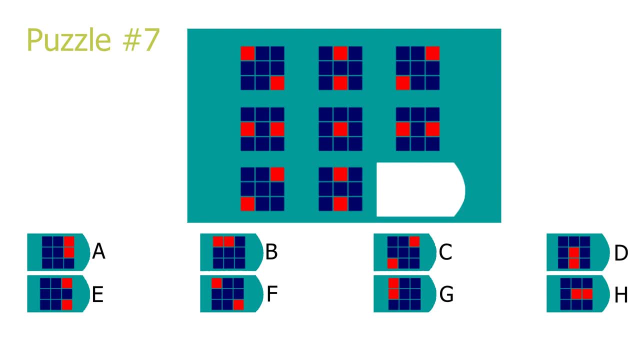 are the two squares which behave differently from each other, but separately they both behave in a predictable way. Let's first look at the top left red square in the first picture. For the columns we have left, middle, right positions. For the rows we have top, middle. 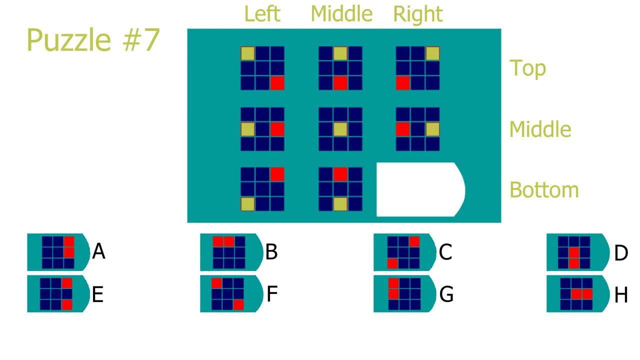 and bottom positions, Leading to a red square in the bottom right corner. If we look at the answers, Only E and F have a red square there, so we can получить all the other answers. Now let's look how the red square in the bottom right corner of the first videos behaves. 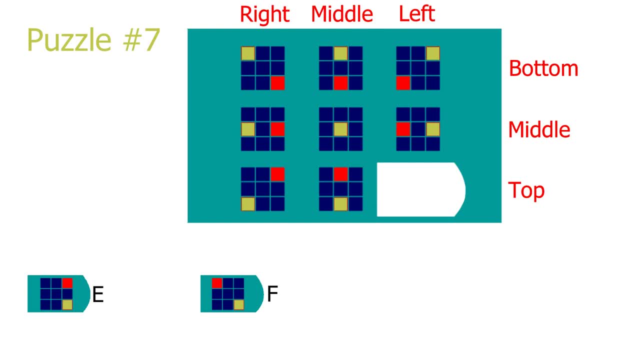 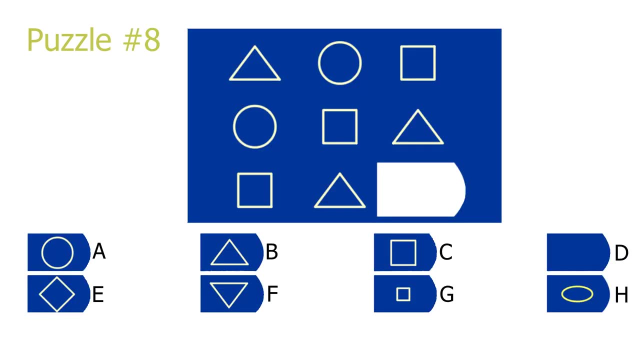 Right, middle, left for the columns, Bottom middle and top for the rows. Therefore, the answer has a red square in the left top corner and the correct answers is F, Puzzle 8.. If we look at the top right towards the bottom left diagonal, we see a repetition. 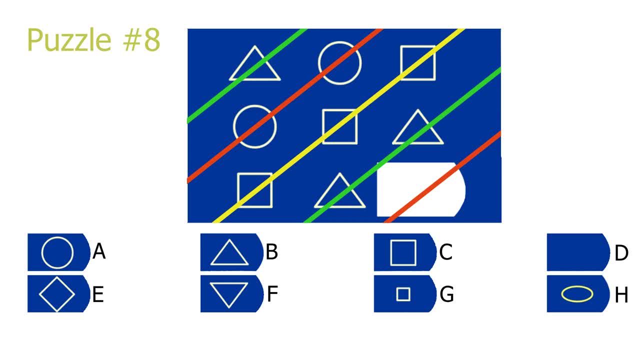 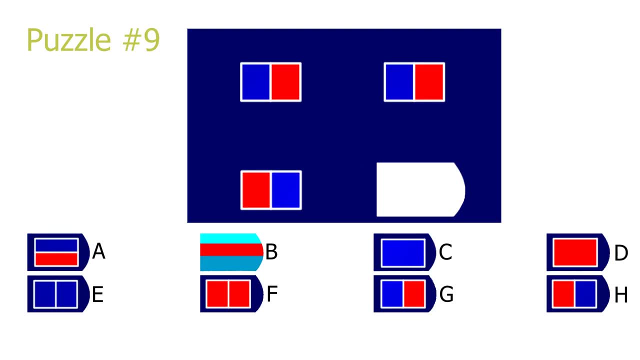 of shapes and the diagonals repeat every three diagonals. Therefore, our answer is a circle and the correct answer is A Puzzle 9.. Another 2x2 puzzle: There is no changes in the rows and there is an inversion of color in the columns, both leading to the answer H, Puzzle 10.. These 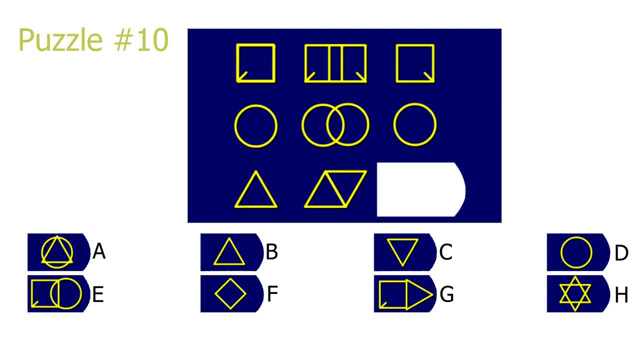 are what I like to call addition puzzles. You take two pictures and add them together in some way. In this example, we have the pictures in the first column added with the pictures in the third column, which creates the second column. If we take a look at the last row, the first picture have a triangle. 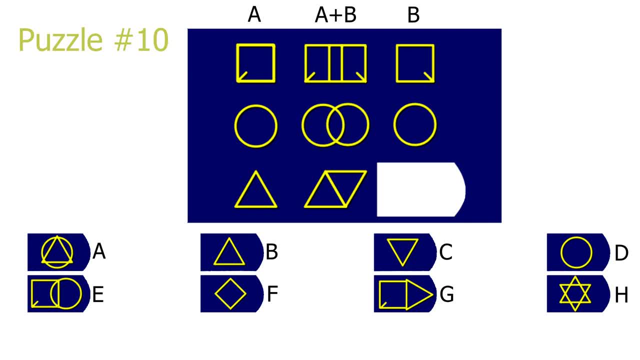 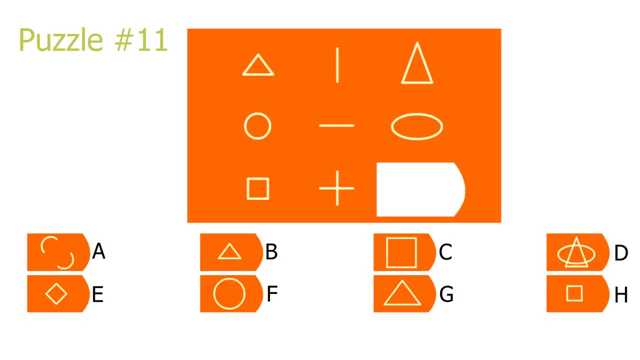 pointing up, and the second picture has two triangles, one pointing up and one pointing down. so our answer has to be a triangle pointing down. C is the correct solution. Puzzle 11. This is a new kind of IQ puzzle I haven't encountered before. These puzzles I will refer to as scaling puzzles. 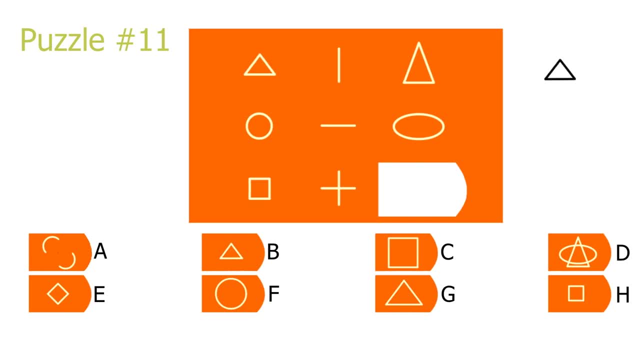 For an example, let's look at the first row. We have a triangle and a scaling factor. The triangle is then scaled up in the direction of the scaling factor and keeps growing until it's as large as the scaling factor. And for the last row, we have a square and a two-dimensional scaling factor. The square is then increased both in. 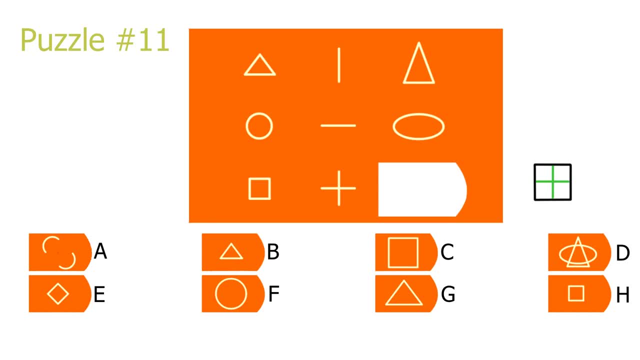 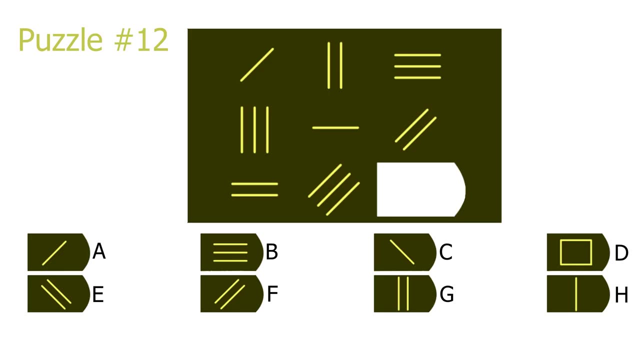 height and width until it's as tall and wide as the scaling factor. This leaves answer C as the correct answer. Puzzle 12. Another diagonal puzzle, but this one goes in both diagonals. If we look at the top right towards the bottom left diagonal, we see the orientation or the angle of the shapes. 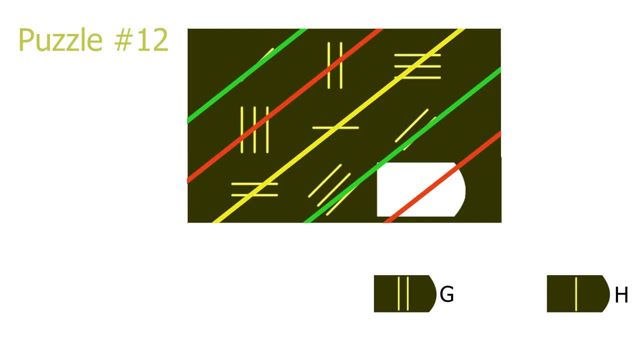 repeats. This leaves only vertical lines as our answer. so G or H. If we look at the top left towards the bottom right diagonal, we see a repetition of the same answer. If we look at the top left diagonal, we will see a repetition of the same answer. This is the correct solution. 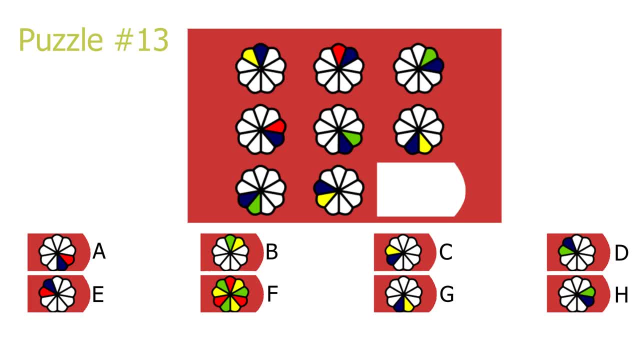 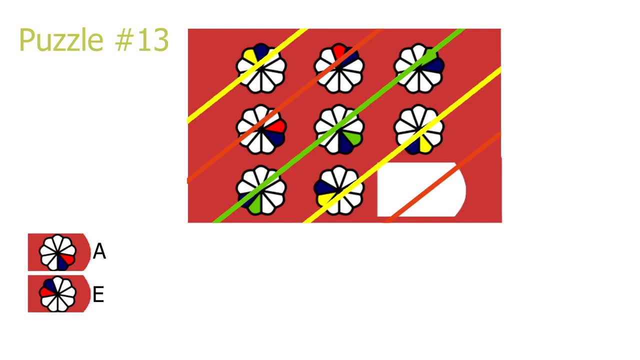 Puzzle 13. This is both a diagonal and a column puzzle. First let's look at the diagonal. from the top right to the bottom left, We have a repetition of color leading our answer to being blue and red, so A or E. For the columns, we have a clockwise rotation of one per diagonal to the right. So if we take 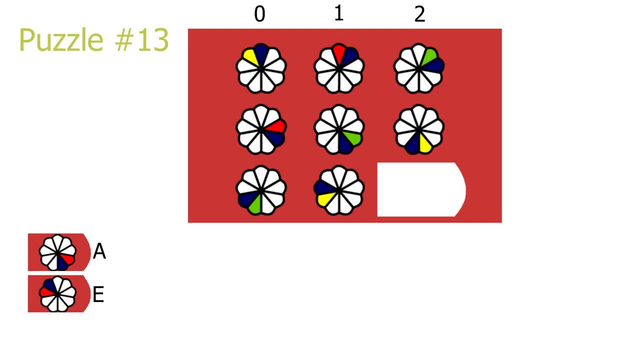 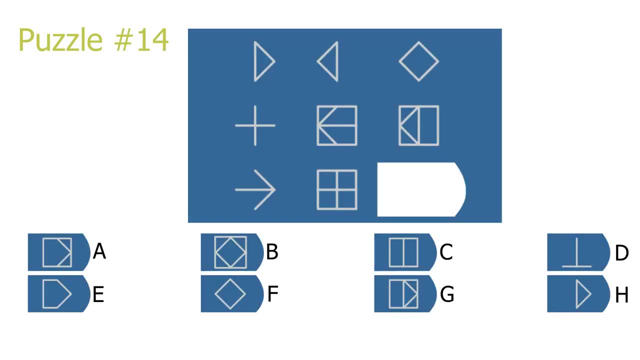 picture eight and rotate the colored areas one square clockwise and then color the yellow area red, get our answer E as the correct solution. Puzzle 14.. Another addition puzzle, but this one involves cancellation as well. If two lines overlaps on an addition, they cancel each other out and become 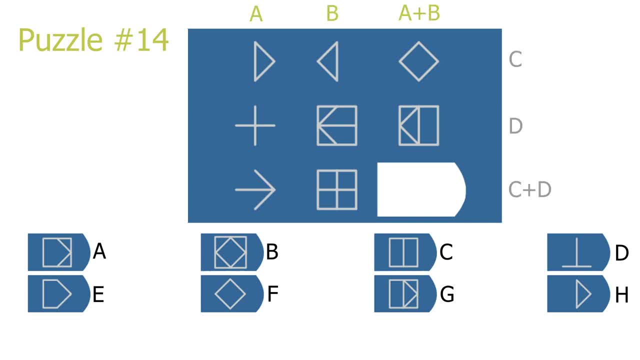 nothing. This puzzle can both be solved on the rows and the columns. Let's go by the columns first. We have a rotated square added with a bigger square that contains half a square with a line running through it. So half the square is cancelled out on the left side and we get. 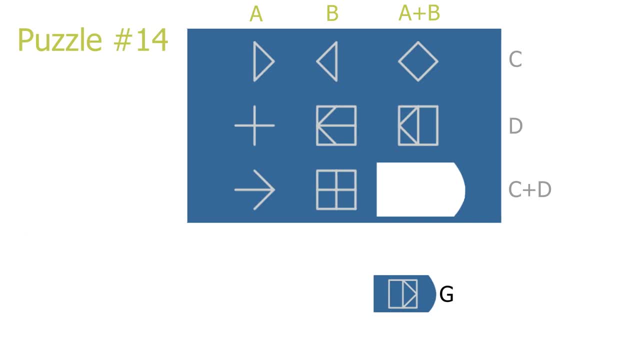 half a square left on the right side, with our line running through it and our bigger square surrounding it. This is identical to G For the rows. the horizontal middle line would cancel out and we would get a simple addition, also leading to G Puzzle 15.. Another addition puzzle, but the. 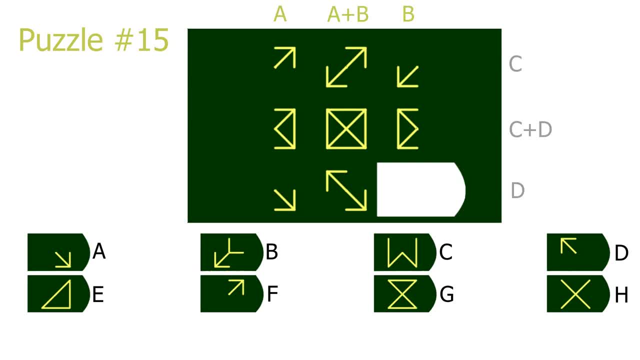 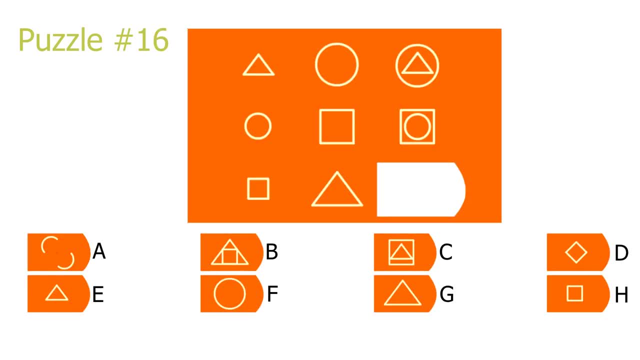 addition is in the middle rows or the middle columns. Again, we can base ourselves on rows or columns, both leading to an arrow pointing to the top left, and our answer is D Puzzle 16.. Another and simpler addition puzzle. This is a simple addition puzzle, but the addition is in the middle rows or the middle columns. This 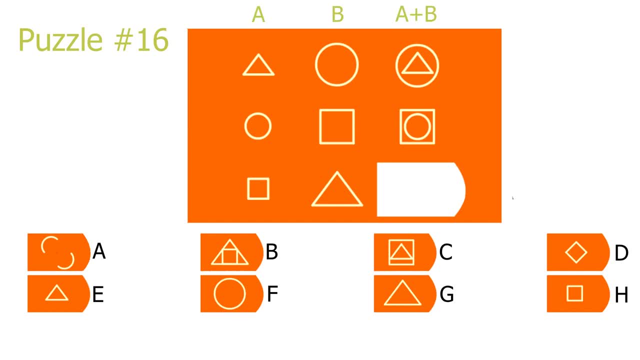 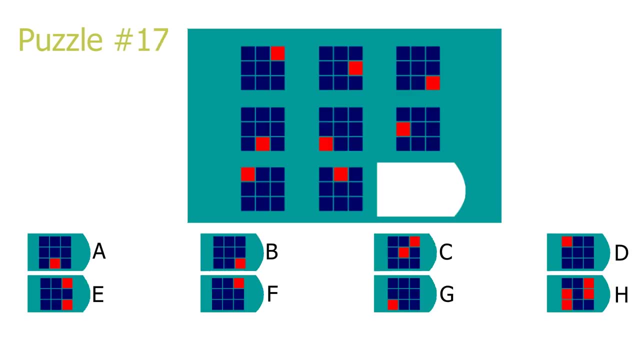 one is only addition in the rows, so the picture in the last column is just the sum of the picture in the two. first, This leads to a triangle with a square inside it, and B is our correct solution. Puzzle 17.. Column arrow puzzle with a red square moving in clockwise direction. In the rows it only. 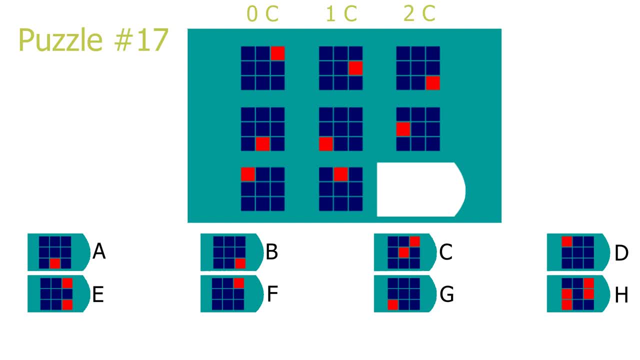 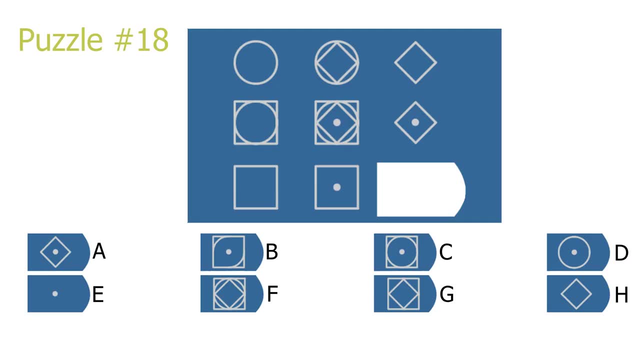 moves one position per picture to the right. So if we base ourselves on picture 8 and move the red square one to the right, we get solution F, Puzzle 18.. Addition puzzle: Middle rows or columns are the sum of the first and third rows or columns respectively. If we base ourselves on the last row, 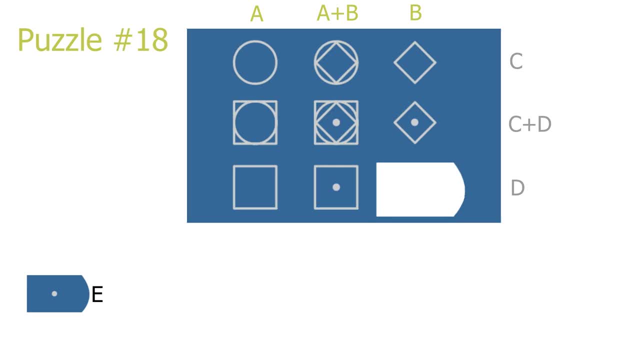 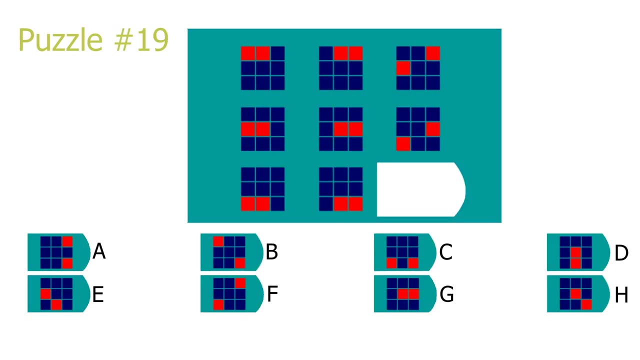 we see quite easily that the answer has to be a dot, So E is the correct solution. Basing ourselves on the last column also leads to the dot Puzzle 19.. The easiest way to solve this is just to go by columns and move the red squares one position down compared to the previous picture leading to. 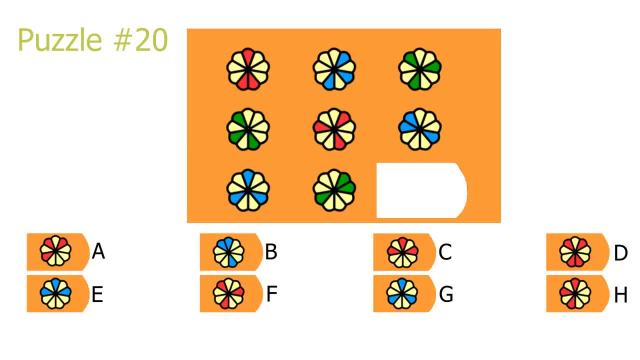 B as the correct answer. Puzzle 20. This is a diagonal puzzle, on both diagonals. Let's first go from top left to bottom right and we see that the first and second rows are the same. We see a repetition of color, So our answer has to be red If you look from top right to bottom left. 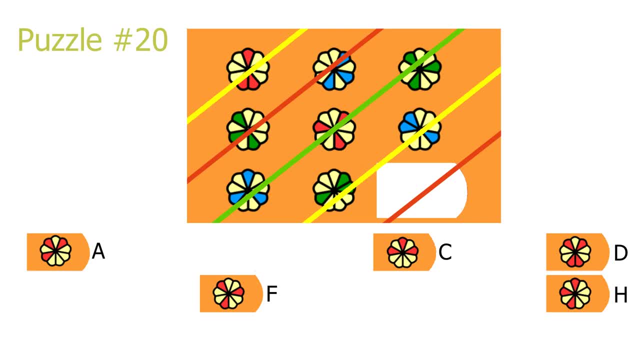 we see a repetition of how many spaces there are between the colored tiles. This leads to our answer being red tile, with one tile separating each colored tile. This leaves answer A, C or H. Now, also looking at this diagonal, we see that the picture in the diagonal sequence always have their colored 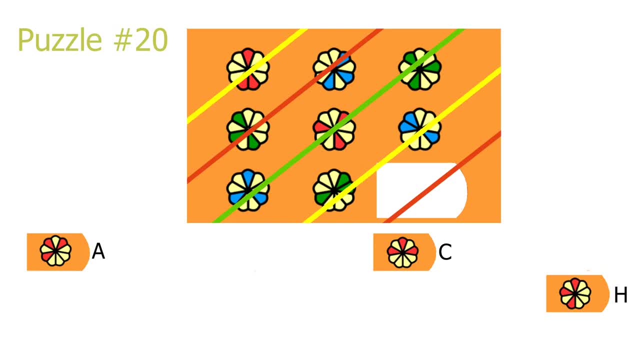 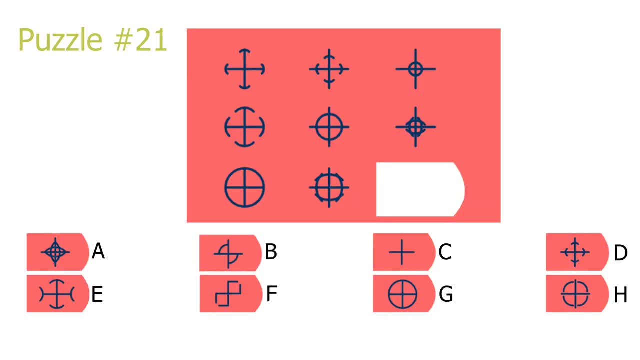 tiles moved, three tiles clockwise per row down. So if we base ourselves on picture 4 and rotate it three tiles clockwise, we get C as the correct solution. Puzzle 21.. This puzzle is based on four circle segments moving towards each other. So we gotta use picture 8 to predict how the 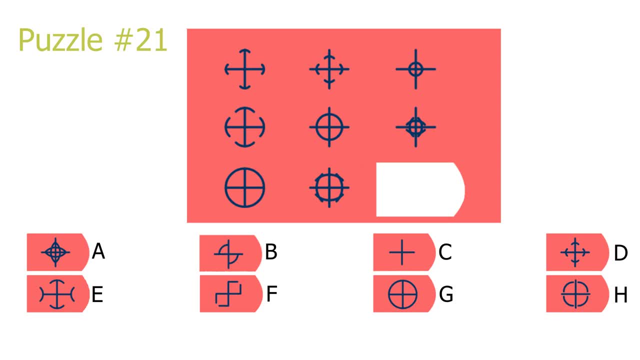 segments will keep going after they keep moving through each other and towards the center of the circle. So we have picture 7 like this, picture 8 like this, and then picture 9 will look somewhat like this, Leading to A being the correct solution: Puzzle 22.. First let's look at the top, right going. 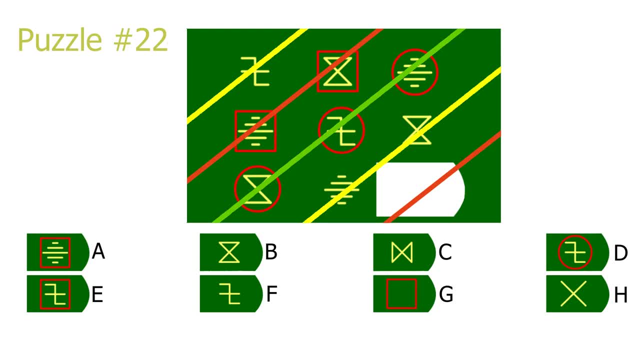 left diagonal And we can easily see how there is a repetition of the outer pattern leading to our answer having a red square around it. This leaves answer A, E or G as correct. In the top left to bottom right diagonal we have a repetition of the inner shape, with the weird C shape in the main. 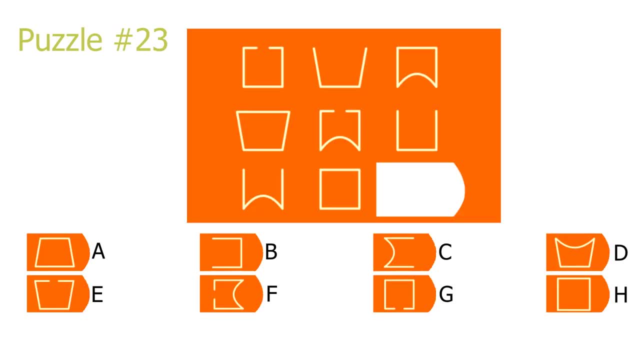 diagonal. So the correct solution is E, Puzzle 23.. Another identical puzzle, Top right to the bottom left diagonal is a repetition of the bottom segment of the picture, leading to a wide shape on our answer. So either D or E will be the correct solution: Puzzle 23.. This puzzle is based on. 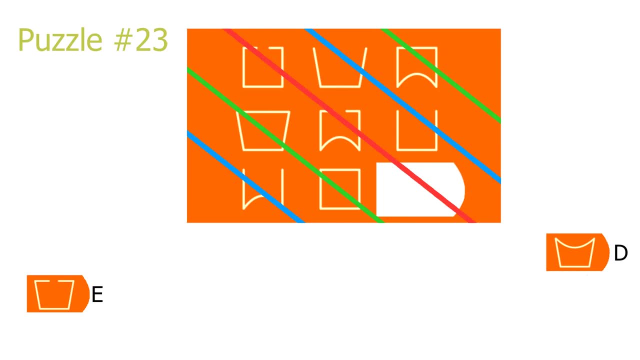 the top right diagonal And we can easily see how there is a repetition of the outer pattern leading to the inner shape on our answer. So the correct solution is E. And looking from the top left to the bottom right diagonal, we have a repetition of the top segment of the picture, which is the 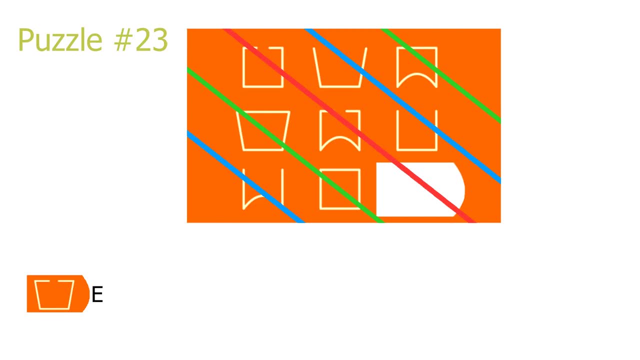 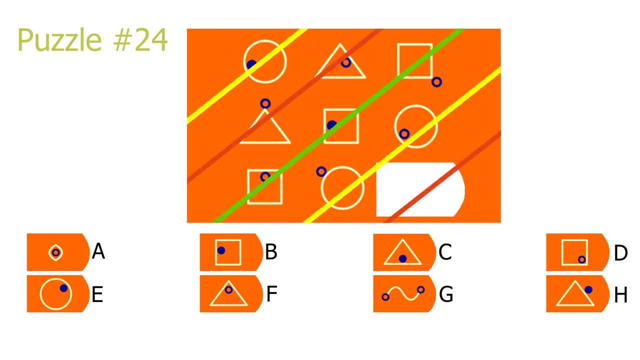 opening in the middle for the main diagonal leading to E as the correct answer: Puzzle 24.. This is the third identical puzzle in a row. Top right to bottom left leads to a repetition of the main shape which leaves a triangle for our answer. So C, F or H is correct Looking at the top left. 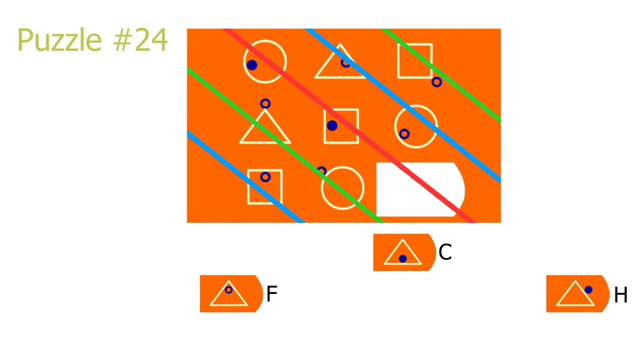 to the bottom right diagonal, we see a repetition of the circles. In one the circles are whole and repeat on the inside. In one they are hollow and repeat on the outside, And in one they are hollow and repeat on the inside. The main diagonal has a whole circle on the inside. 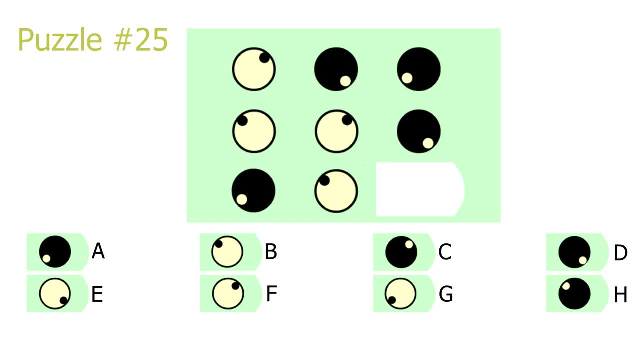 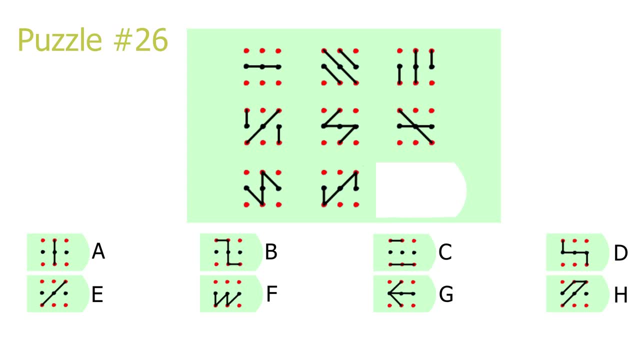 leading to C as the correct answer: Puzzle 25.. There is a repetition on the top left to the bottom right. diagonal F is correct: Puzzle 26.. This is a very interesting puzzle. I liked it very much. So we have three different points of rotation which have some line attached to them. 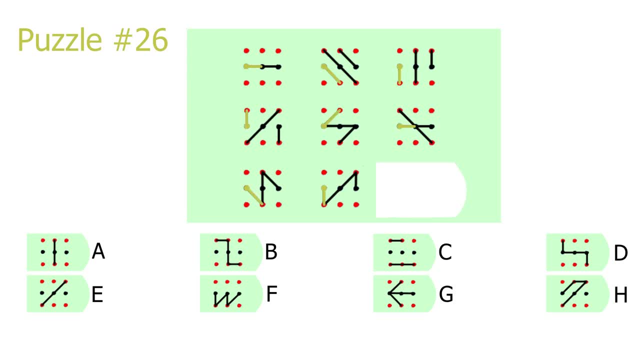 and they rotate by some rules: Puzzle 26.. You have three different points of rotation which have some. First, let's go by the middle left dot in the first picture. Moving down the rows, they just move one dot clockwise. and moving down the columns, they just rotate two dots counterclockwise. 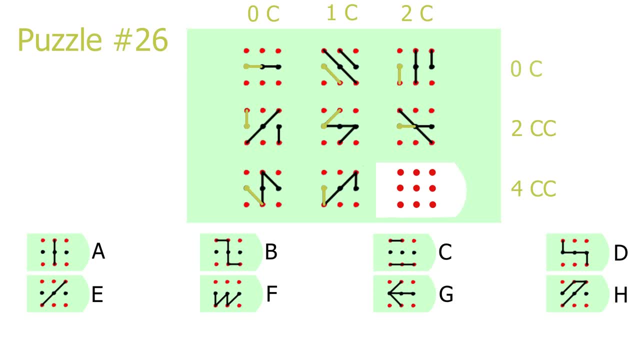 So if we have our answer here, we can see how the middle left dot rotates one dot clockwise in the rows leading to this angle, or how it rotates two dots counterclockwise in the columns leading to the same answer. Okay, we're done with the one on the left in the first picture. Let's go by the middle one. 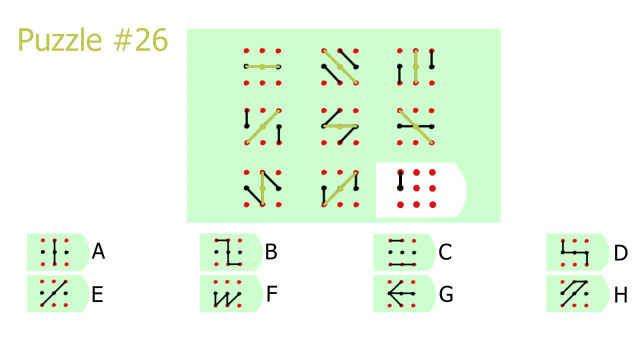 This dot has two lines pointing in opposite directions of each other. For the rows, we have one clockwise rotation per move to the next column. For the columns, we have one counterclockwise rotation per move to the next row, both leading to a horizontal line as our answer. 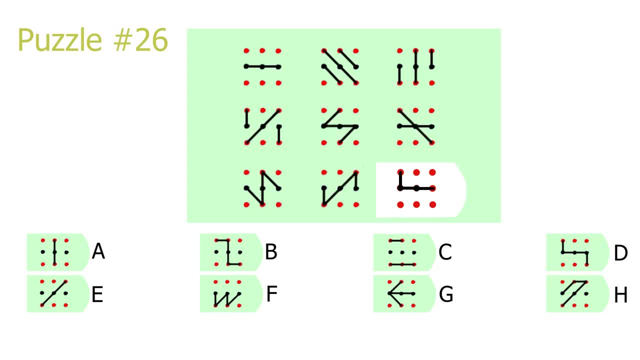 So actually just knowing the rotation of the first dot was enough to solve the puzzle, but I think just explaining the full derivation of the answer is better. Last dot on the right in the first picture: This one actually has two lines pointing in opposite directions of each other. 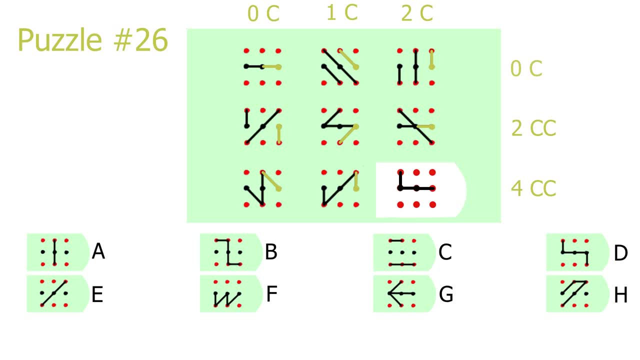 This dot has the same rotation as the first dot, but just different starting positions. Let's just go by the last column and rotate it two positions counterclockwise and we end up with a line pointing straight downwards. D is the correct solution. 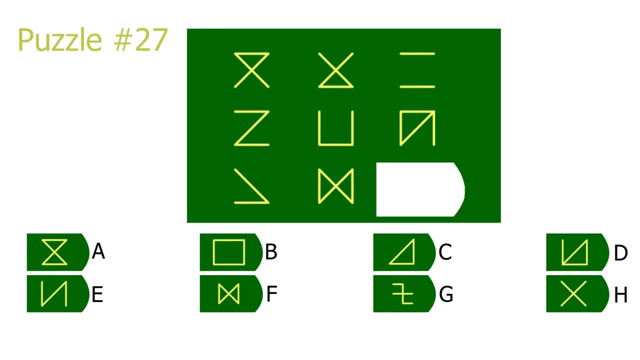 Puzzle 27.. This is an addition puzzle with cancellation. If we base ourselves on the rows, we see that the first picture adds with the second picture and if we go by the columns, we see the exact same thing. The first picture adds with the second picture to create the third picture. 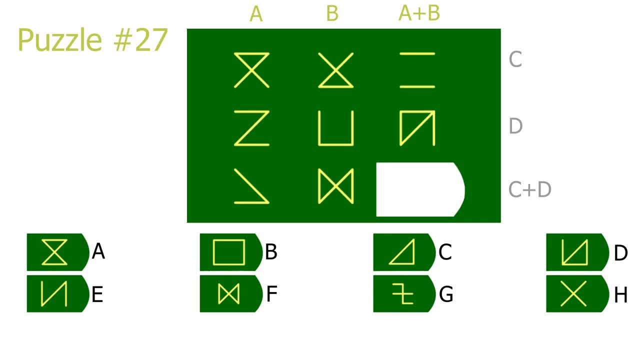 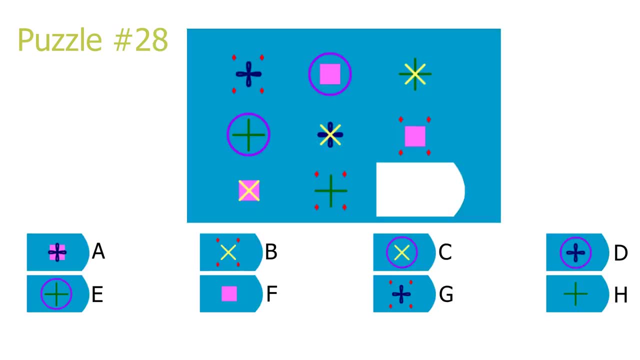 Basing ourselves on the third column, we see that the line on top cancels each other out and we just have picture 6 without a top and with a bottom. So D is the correct solution. Puzzle number 28.. This is a diagonal puzzle on both diagonals. 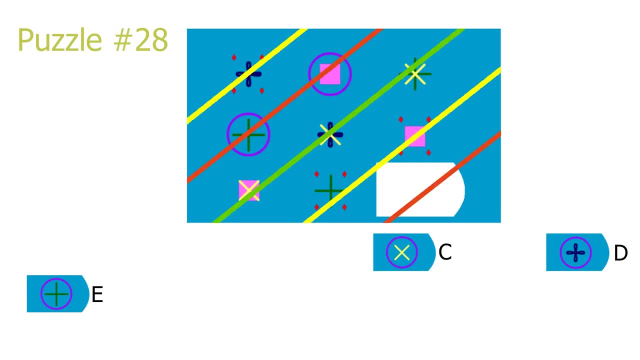 Top right to the bottom left diagonal leads to a purple circle in our answer, leaving C, D or E as the correct answer. Top left to bottom right diagonal leads to a repetition of the middle shape, which is a blue cross in the case for the main diagonal. 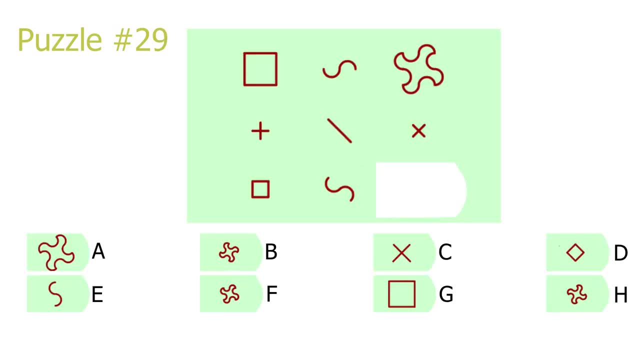 D is the correct answer. Puzzle 29.. This is another scaling puzzle with a new concept which is rotation of the scaling factors. So we can see by the columns that the last picture is just the first picture, just scaled down or rotated by some degrees, which is described by the scaling factor in the middle. 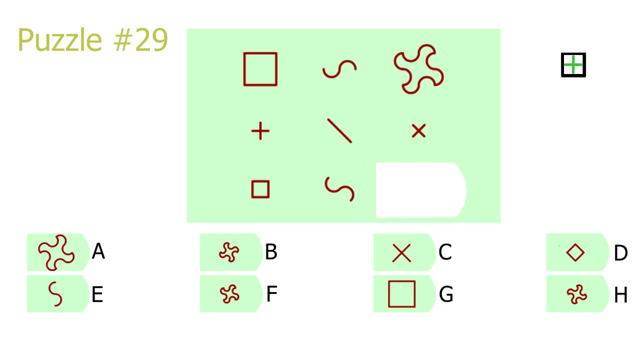 Let's do an example: Big box, small scaling factor, small box And for our answer we have a big drawing star with a small scaling factor. So we take the big star, update the small scaling factor and we scale it down. 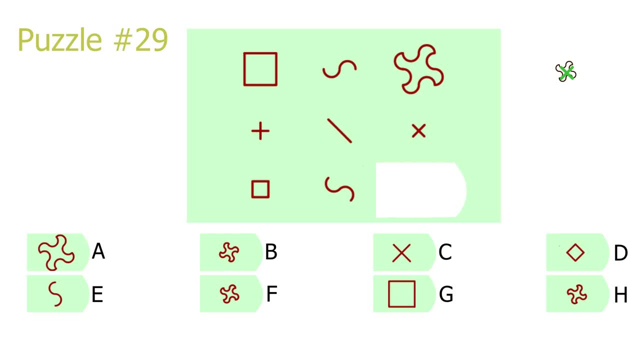 But we also see that the scaling factor has a 45 degrees rotation counterclockwise. so we just have to rotate our picture 45 degrees counterclockwise to make it identical to the scaling factor. I'll just add a picture above so you can see it better. 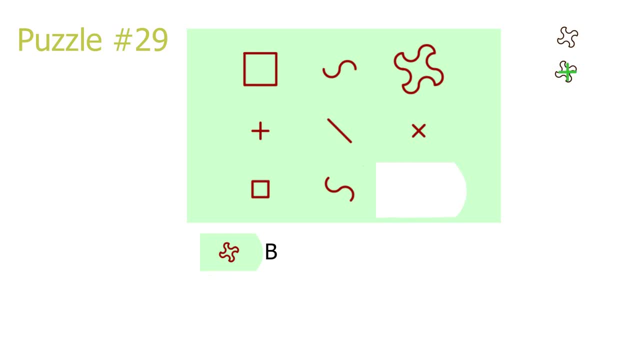 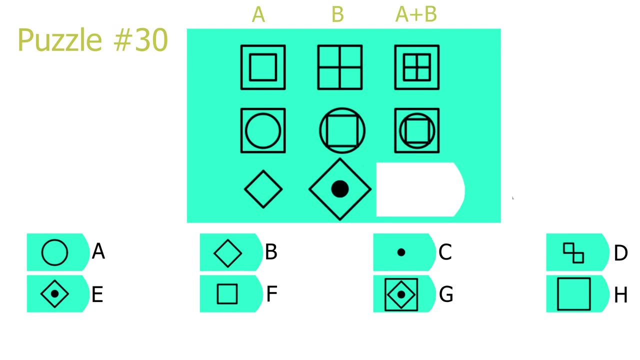 So we rotated 45 degrees counterclockwise And of course B is our answer. Puzzle number 30.. This is a mixture of addition puzzle and scaling puzzles. The pictures in the middle column is scaled down to fit inside the smaller shape in the pictures in the first column. 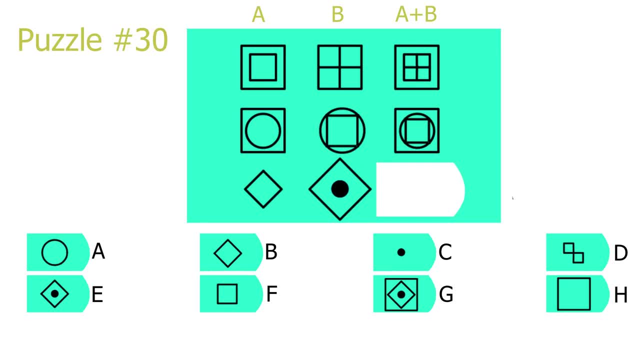 and then they're added together to produce the pictures in the third column. So for our answer, we take picture 8, scale it down to fit inside picture 7, and then add them together and we get E as the correct solution. 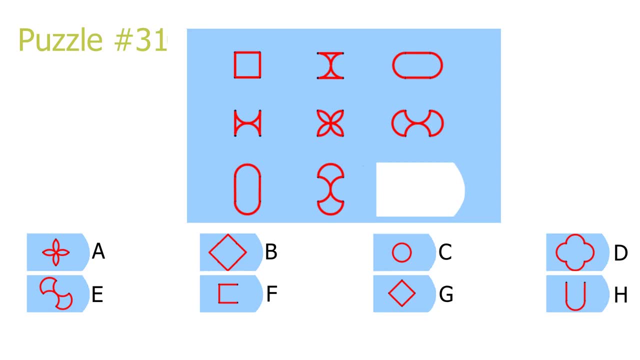 Puzzle 31.. So this is an addition puzzle in disguise. So if we just normally add picture 1 and 2 together, we have some area which is not overlapped by both of them. This area is then mirrored over the lines of the square. 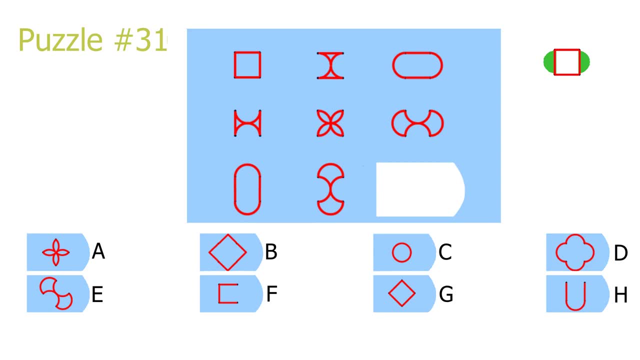 Now we just remove picture 1.. So we take picture 1 and 2 and add picture 1, and then we draw around the area which was not overlapped and then remove the insides leading to the last picture. This works for every row and every column in this picture. 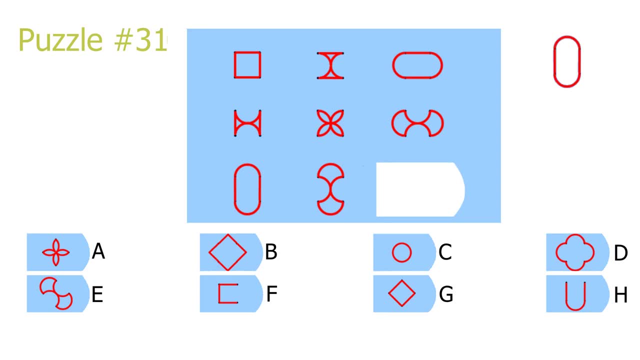 Let's look at the last row to get an answer. So the same steps to get the mirrored area. We draw around it and then we remove the inside, leading to picture D as the correct solution, Puzzle 32.. This is a one column puzzle. 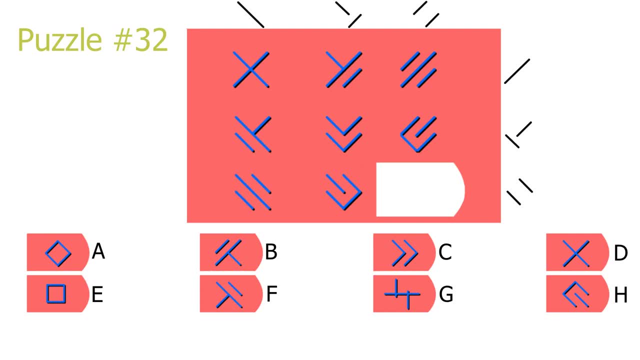 So our first column has two diagonal lines going from top left to bottom right. Our second has one diagonal line going from top left to bottom right and one diagonal line going from top right to bottom left. The last one has two diagonal lines from top right to bottom left. 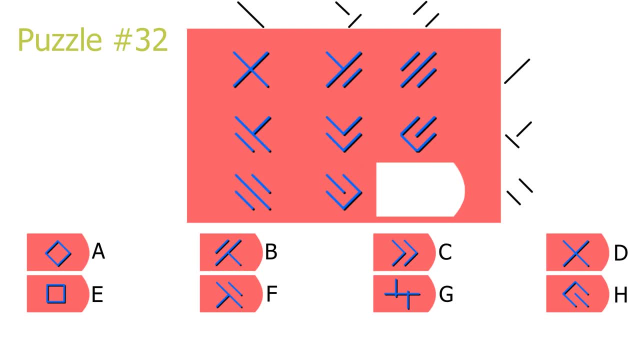 Keep in mind that these are all in the same position, so in the top left and the bottom right And for the rows we have in row 1, two diagonal lines from top right to bottom left. In row 2, we have one diagonal line from top right to bottom left. 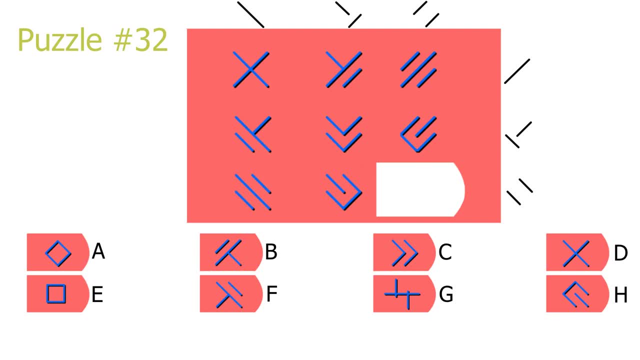 and one diagonal line from top left to bottom right. And in row 3, we have two diagonal lines going from top left to bottom right. Keep in mind that these are also in the same position, which is top right and bottom left. So just adding the last row and last column together. 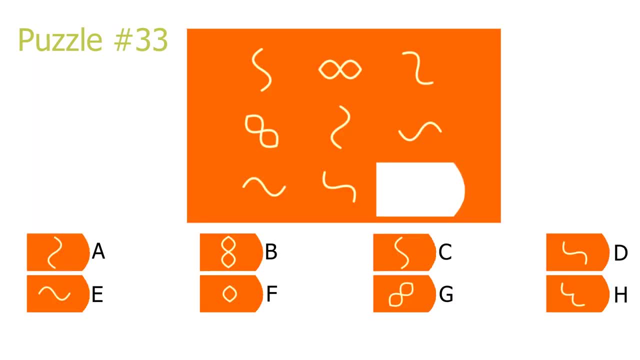 we get a diamond shape, which is our answer, A Puzzle 33.. This is just a simple diagonal puzzle. on two diagonals- Top right to bottom left diagonal. we see a repetition of shapes and our answer has to be a double helix shape. 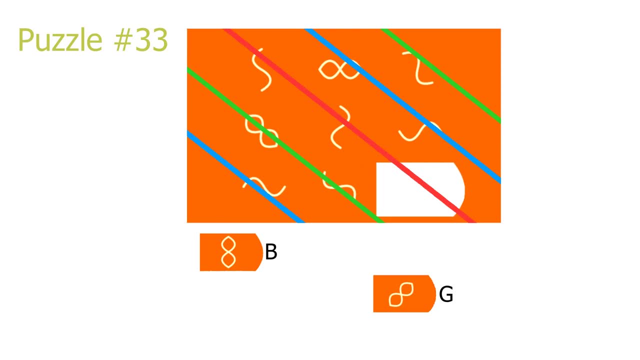 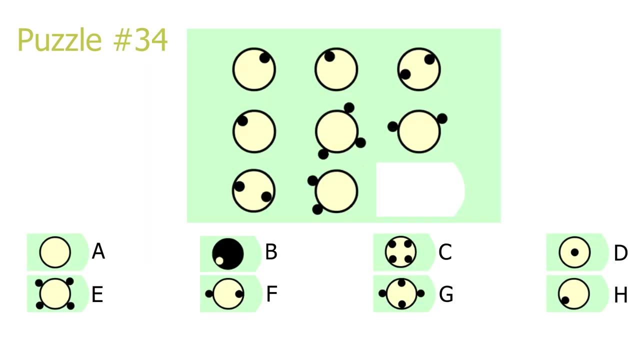 Top left to bottom right diagonal. we see all the shapes point in the same direction. So our answer has to be vertical and B is the correct solution. Puzzle 34. This is an addition puzzle with a twist. So in this puzzle we just have some white circles. 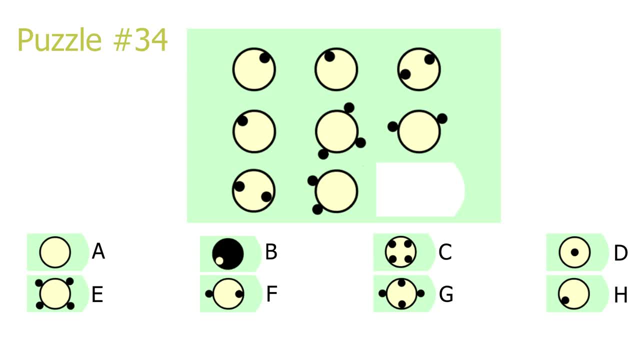 which have black circles either inside them or outside them. If we look at the first row, we see how the black circles inside the first picture and the second picture add together and produce two black circles inside the circle of the final picture And in the second row. something else is happening. 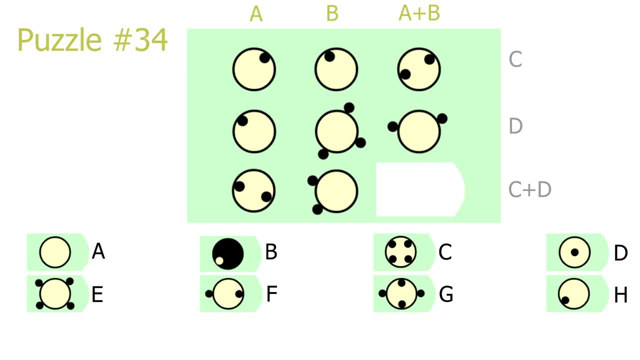 The black circle inside the circle in the first picture cancels out one of the black circles outside the circle in the second picture. This leaves two black circles outside the circle in the third picture And, of course, by the last row, we have two black circles outside and two inside. 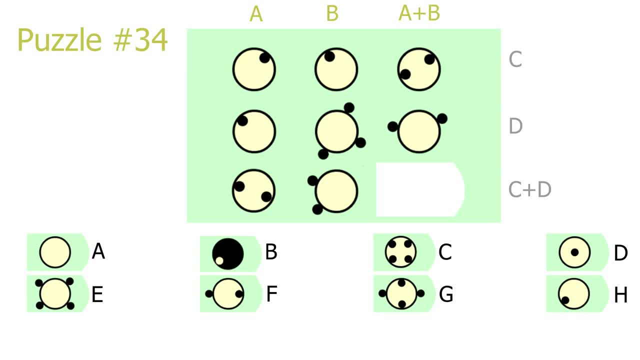 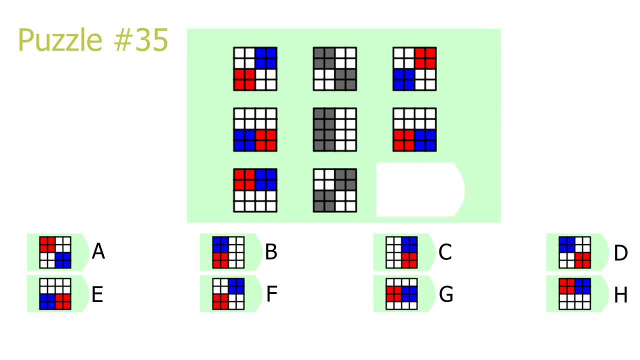 which leads to a full cancellation. So our answer will just be a white circle, and A is the correct solution. Puzzle 35.. This is a row puzzle with similarities to our factor puzzle. The middle column describes the mirroring between the first picture and the third picture. 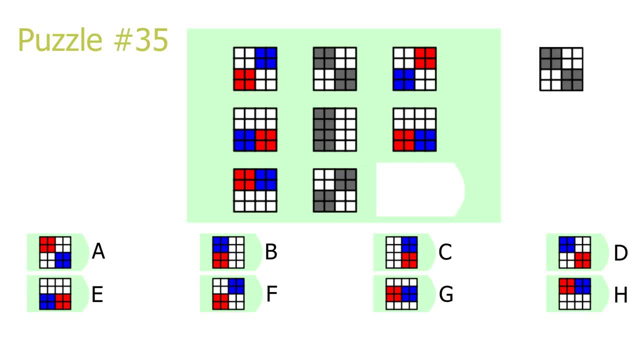 For example, we have the first row. We have this mirror factor which is equivalent to a line going across the diagonal from top left to bottom right. Now if you place this on picture one and mirror it along that diagonal, we get picture three. 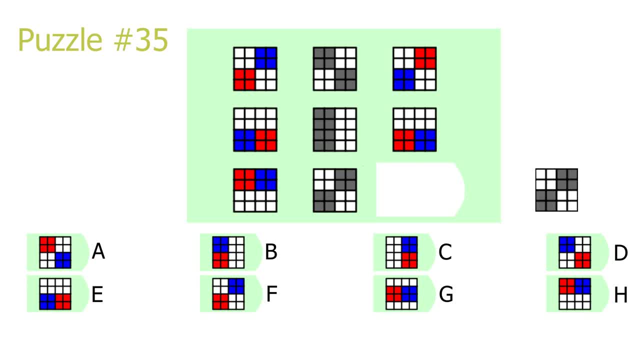 So for our last row we have this mirror factor equivalent to a line going across from top right to bottom left. Place it on top of the first picture in the row and mirror it across the diagonal to get picture C. C is the correct answer. 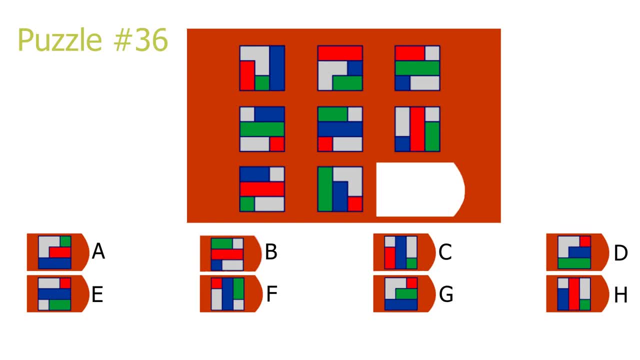 Puzzle 36.. A diagonal puzzle with several rows across the same diagonal. So if we look at the top right to the bottom left diagonal, we see firstly that the way the picture points is always the same for every picture in the diagonals leading to a picture. 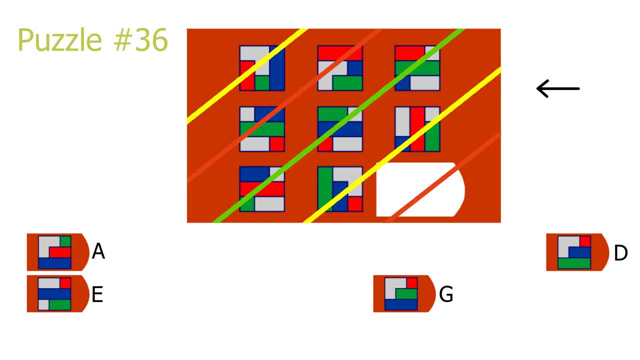 pointing from right to left. This leaves A, D, E or G as the solution. And secondly, we can see that the colors change in a specific pattern across the diagonal. I'm talking about the colors of the rectangle of a specific length and I'm not talking 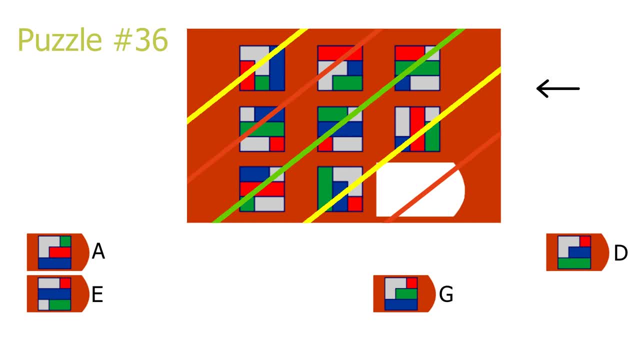 about the position of these rectangles. So if we look at the rectangles of same length across the same diagonal, we see that it changes in a way that red becomes green, green becomes blue and blue becomes red. Using these rules, on the fourth picture we see that the big triangle has to be blue. 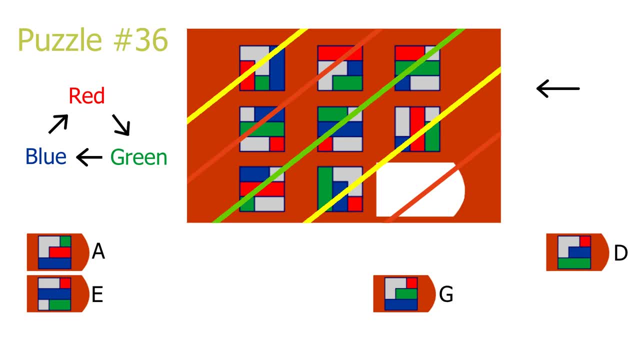 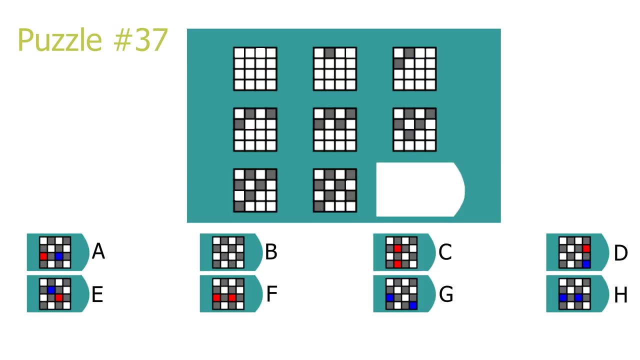 the medium triangle has to be red and the small triangle has to be green. These colors only match A, so A is the correct solution. Puzzle 37.. Just quickly to see the obvious pattern, I'll remove the colored tiles. We see how they're added from left to right, filling two by two squares at the time. 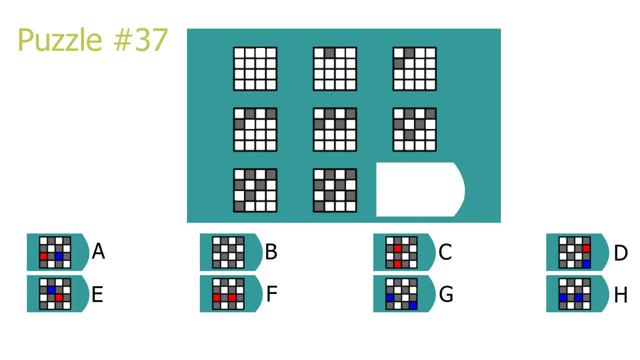 first in the top right, then in the bottom left and moving towards the right and repeating. So our answer will have a gray pattern, kind of like a chessboard pattern, alternating between white and gray. So now we have to figure out how the colored tiles move. 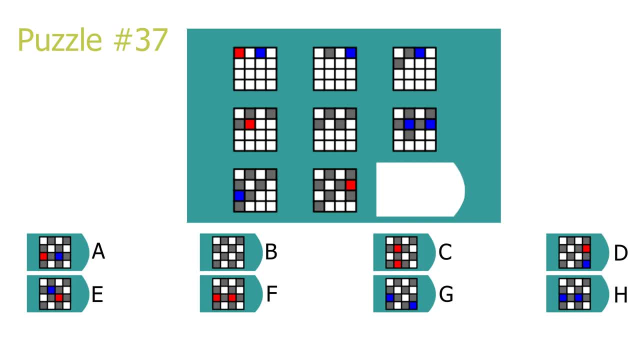 Now imagine that the two colored tiles in the first picture is the same for all the colored tiles in all the pictures. They're moving one towards the right in each picture. When they reach the edge of a picture, they pop up again on the row below it. 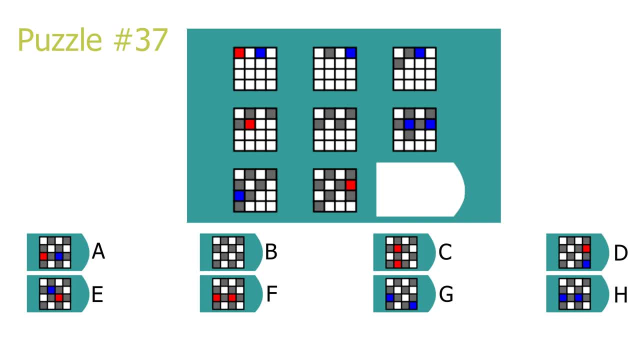 in the most left position. Now, the reason they do not appear in every picture is because the gray tiles sit on top of them and blocking them from you. So those are the basic rules on how the squares move, But we have to ask ourselves how do they change their colors? 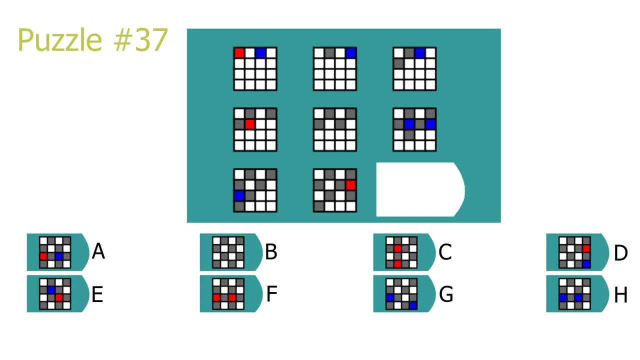 Every time a blue tile goes under a gray tile, it becomes a red tile, and every time a red tile goes under a gray tile, it becomes a blue tile. Hopefully you can see all of this movement and changing of color as they move through. 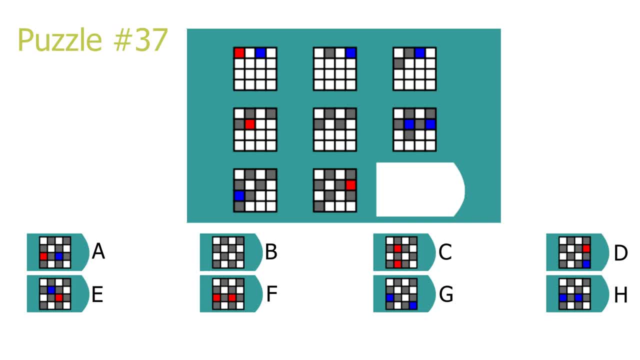 the picture, starting in picture 1 and following all these rules, to picture 9.. So by looking at picture 8, we can see that the red tile is about to move outside the square where it will teleport to the row below in the left, most position. 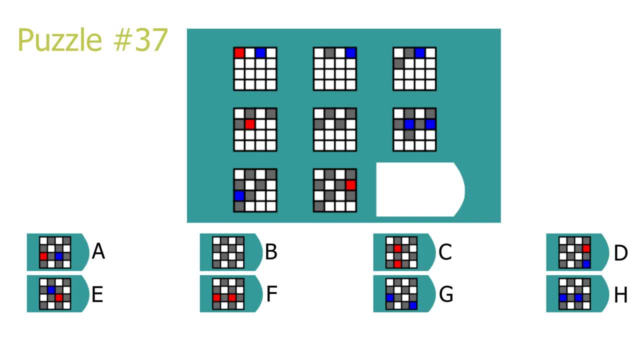 So the answer will have to have a red square in the third row and first column, Leaving A or F as the correct solution. At picture 7 we see a blue square moving under a grey square, going to picture 8, where it changes to become a red square. In picture 9 it will appear as a red square in the third row and 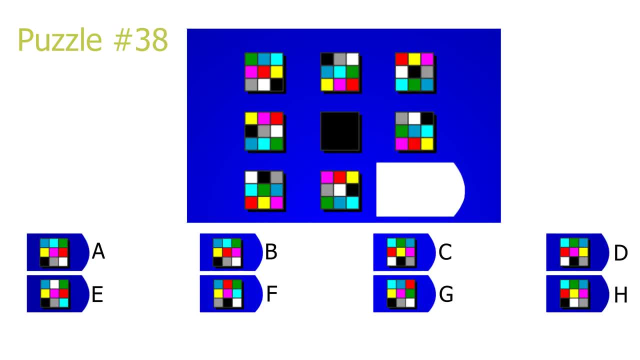 third column leading to F as the correct answer. Puzzle number 38.. At first this puzzle may seem a bit overwhelming, with all the colors to keep track of, but it's a fairly easy puzzle. All you have to do is just to focus at one color at a time. We see that in every row and column. the 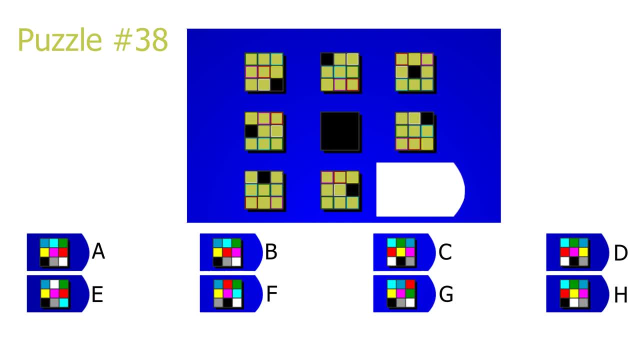 black tiles appear once and only once in every row and column of the pictures. So, looking at the first row, we have a black square in the last row and last column. In the second picture, we have a black square in the first row and first column. So this means that in our last square we have to. 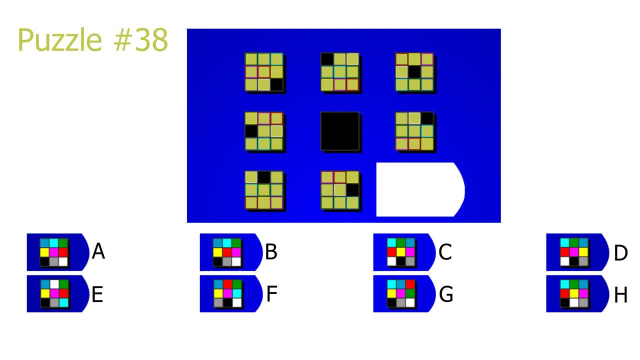 have a black square in our middle row and middle column. So applying this to the last row leaves a black tile in the last row and first column. If you look at the answers, A, B, E, G and H have a black square in the bottom left corner. 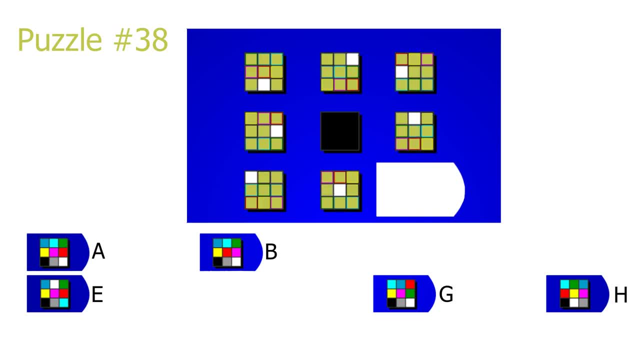 Let's find a new color. Let's pick white. Again, the same rules. We can derive that there is a white tile in the third row and third column. So if you look at the answers, that leaves only A, B and G with a white square in the bottom right corner. Before just wasting time trying a new color, let's 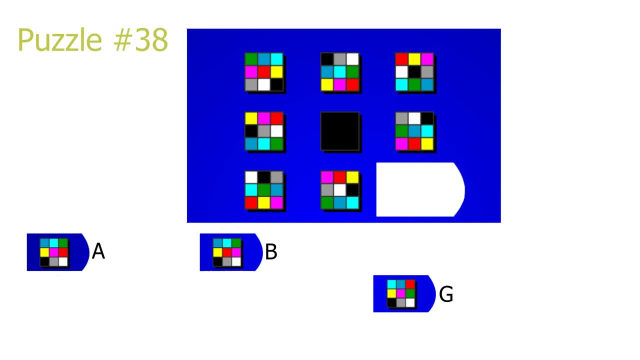 look at the answers, We have to ask ourselves: is there any color which is not similar in every picture? And yes, there is. Red is not common for any of the answers. So let's see what position red should be in and we can derive the solution. So we see that the first row and last row is taken. so 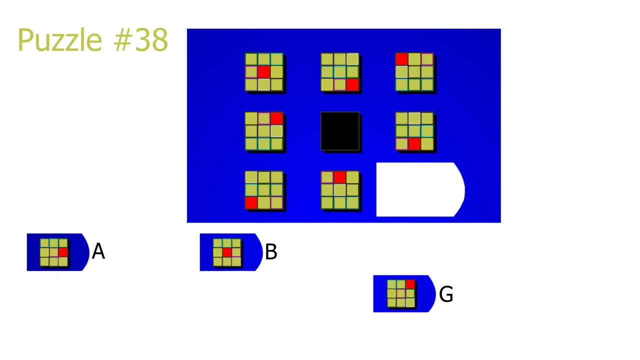 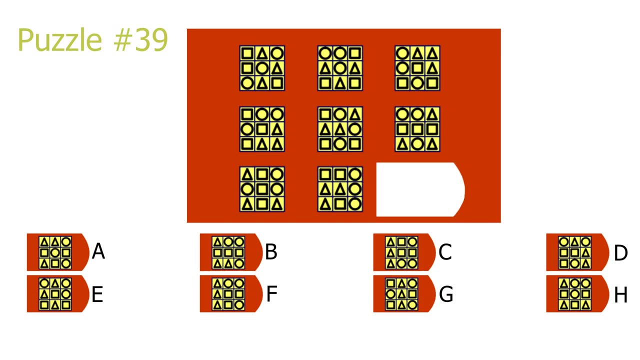 it has to be in the middle row and we see that the first and second column is taken. so it has to be in the last column, And we get that A is the correct answer. Puzzle number 39. The final puzzle. So after looking at this puzzle for some time, one thing caught my eye. There is a repetition of 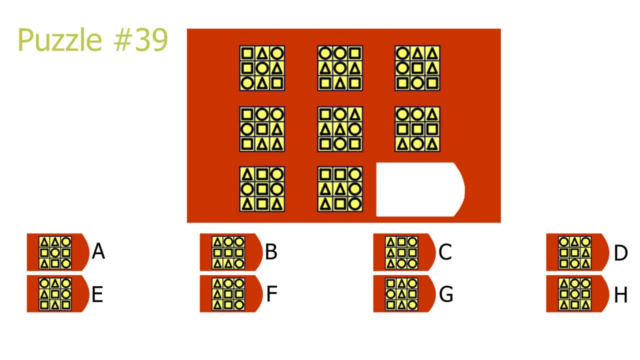 three squares and three circles in the last row It seems to move towards the right. Now, if you look at odd squares on odd pictures, Do all squares become circles and move one to the right? Well, actually no. But if you look only at,